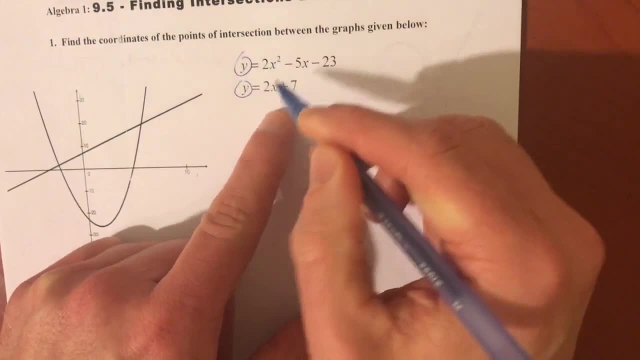 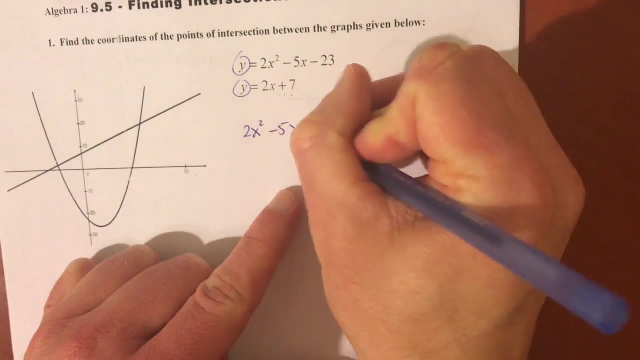 they're equal. I set these two things equal to each other. It's really just substituting this in place of y. So take these two equations. whenever you want to know where two graphs intersect, take their two equations and set them equal. When does this equal that? 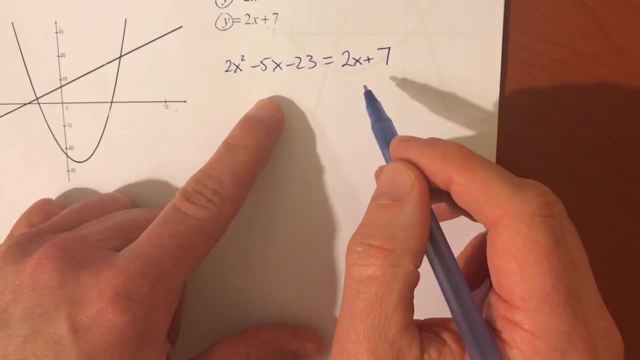 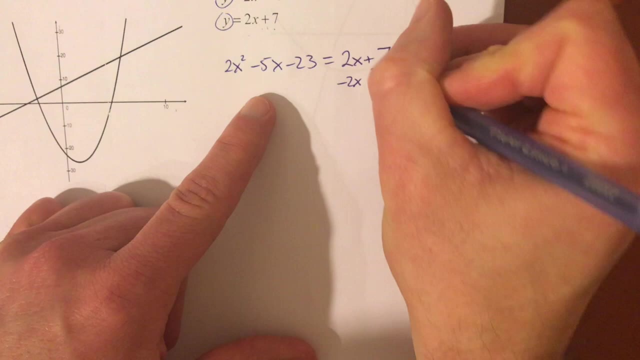 And now you see, we're just solving an equation, like we've been dealing with the last couple days. so we're going to get everything on one side. we're going to be a hero, make it equal to zero. so I'm going to subtract 2x, I'm going to subtract 7.. 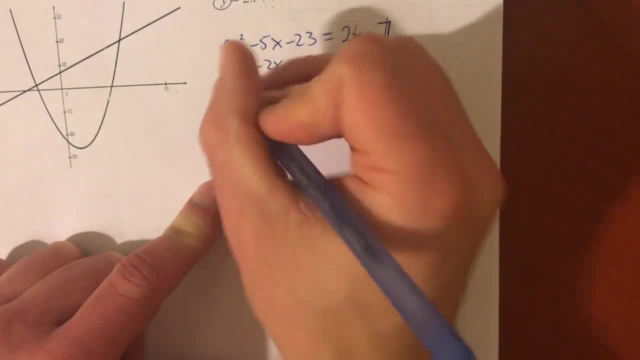 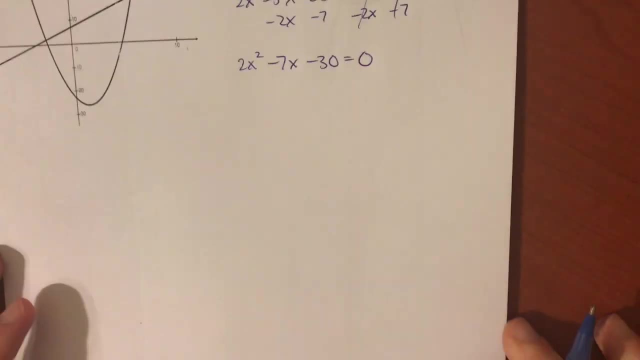 And now that's going to give me a new equation which says: 2x squared minus 7x minus 30 equals zero. And I cannot factor this thing. there's no GCF and it's 2x squared, not x squared. 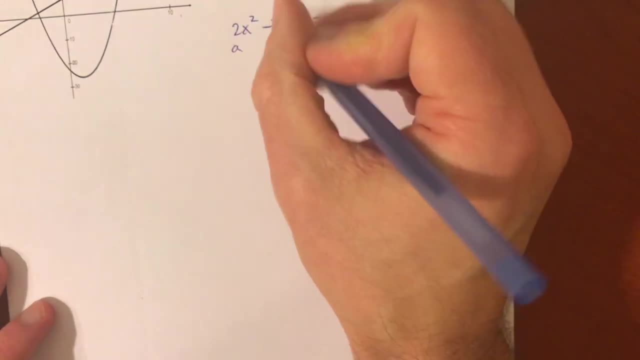 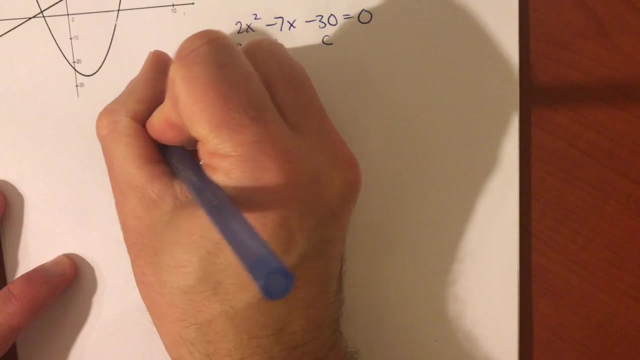 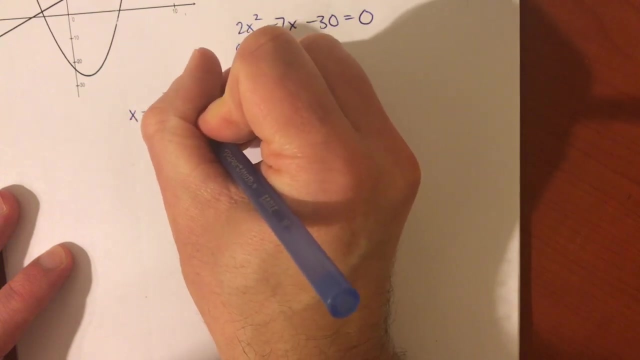 so it's time for that old quadratic formula: A is 2,, B is negative 7, C is negative 30. So here we go: X equals- And we may as well sing it- X is equal to negative B. so that's 7, plus or minus the square root of B squared minus. 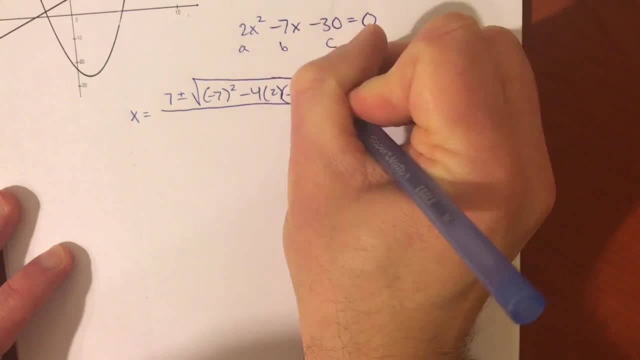 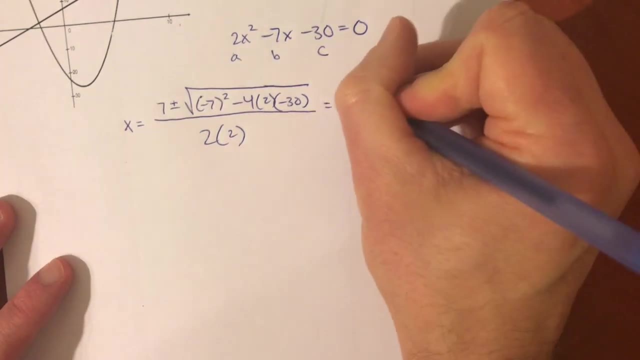 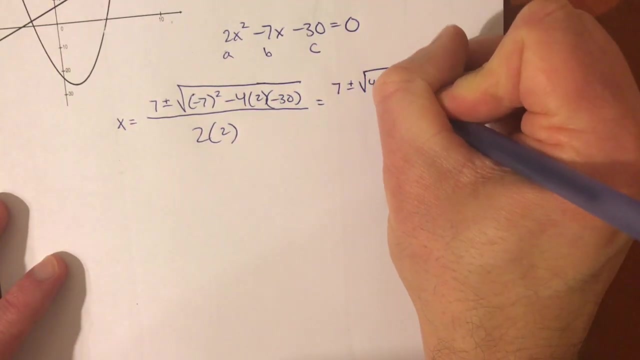 4ac all over 2a. And now we just take our time and simplify this and we're rolling here. So that's 7 plus or minus. the square root of negative. 7 squared is always going to give me a positive number, 49.. 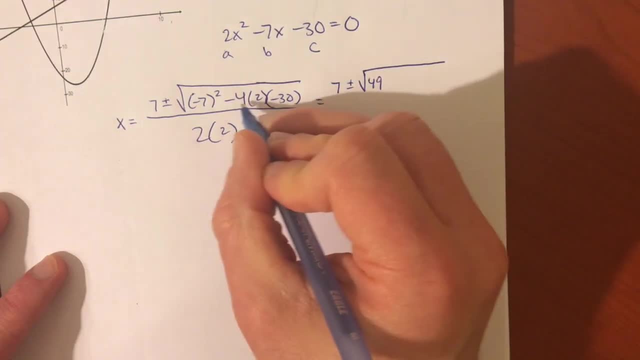 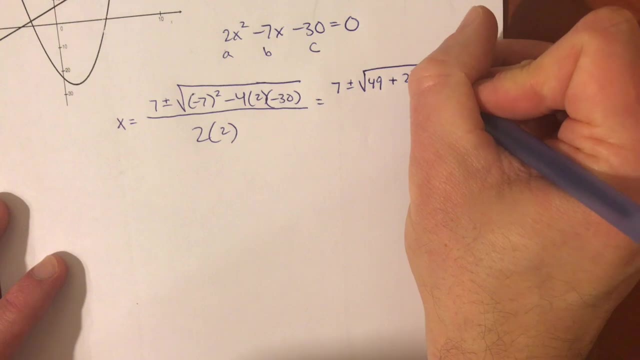 Negative 4 times 2 times negative: 30.. Negative times positive times negative. that's positive 4 times 2 is 8.. 8 times 30, that's 240, all divided by 2 times 2, which is 4.. 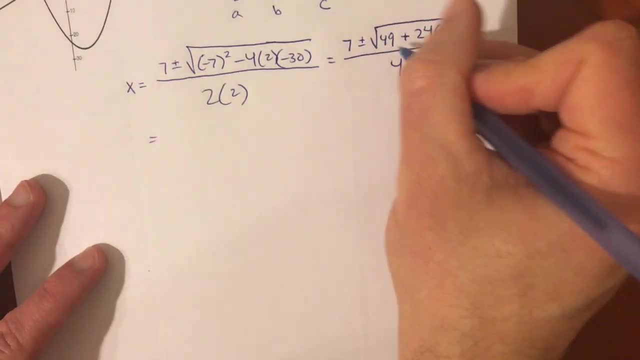 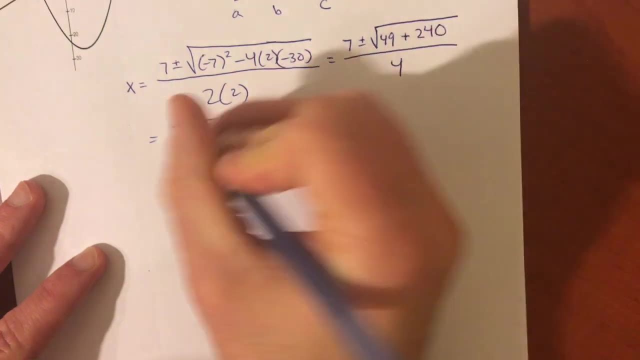 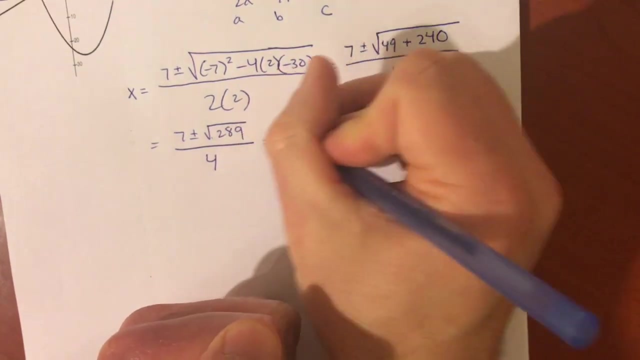 Add that inside. Remember, don't divide by 4,, really, until you've dealt with the square root completely And you get 289, all divided by 4.. And when you go and take the square root of 289 on your calculator, you will notice that. 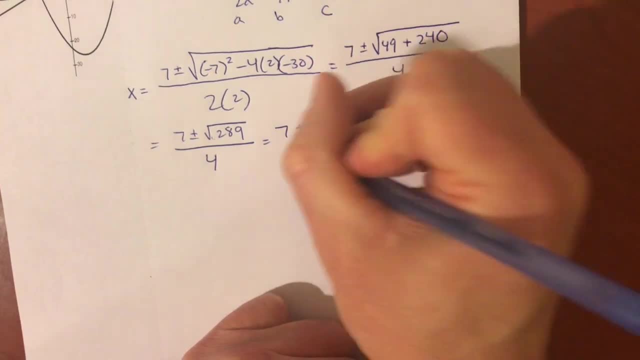 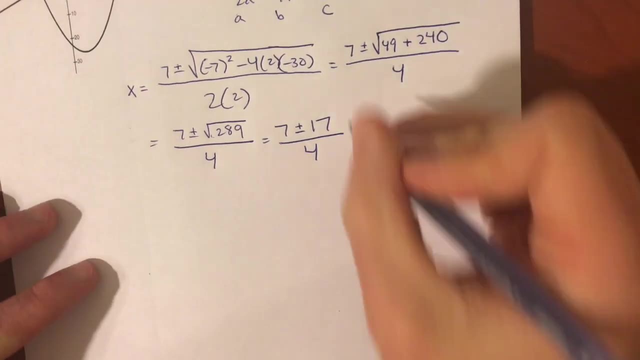 it's a perfect square. The square root of 289 is 17.. So our answers are actually going to be rational, no decimals needed, But it still does give you two answers. remember, be careful. That means 7 plus 17 divided by 4.. 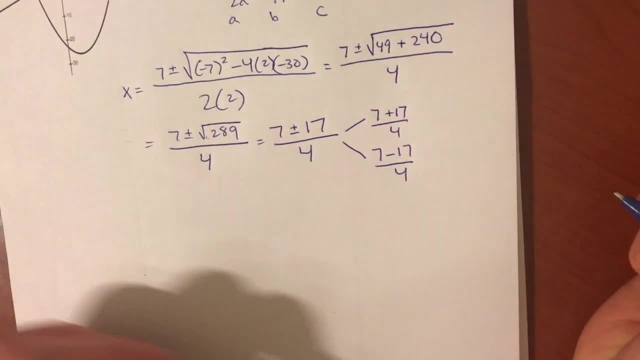 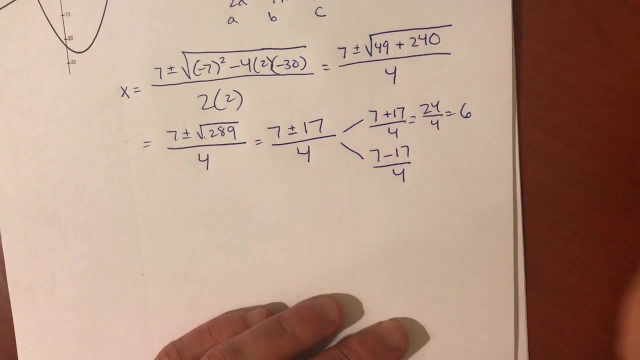 And 7 minus 17 divided by 4.. 7 plus 17.. That's 24, divided by 4, 6.. 7 minus 17,. that's negative 10, and divided by 4, that is not an integer. 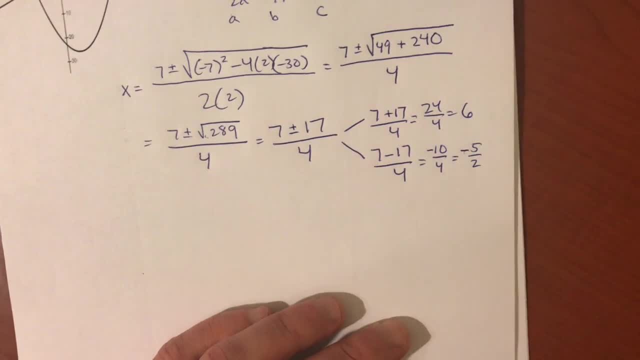 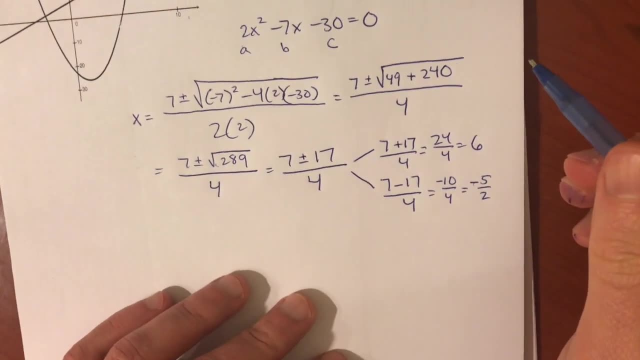 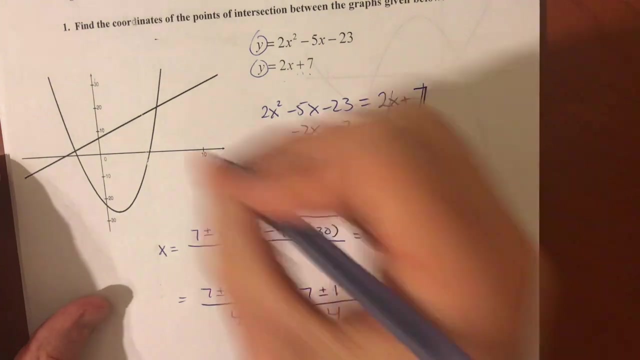 We get negative 5 halves, Or negative 2.5, if you want to use a decimal. The only difference here is that they are asking for the coordinates of the points of intersection. So, just like when we did systems of equations, you were finding coordinates where they intersected. 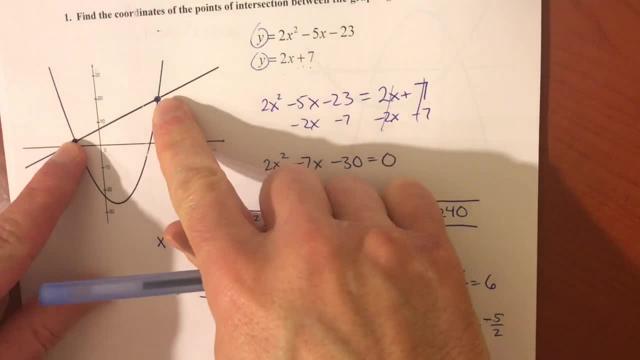 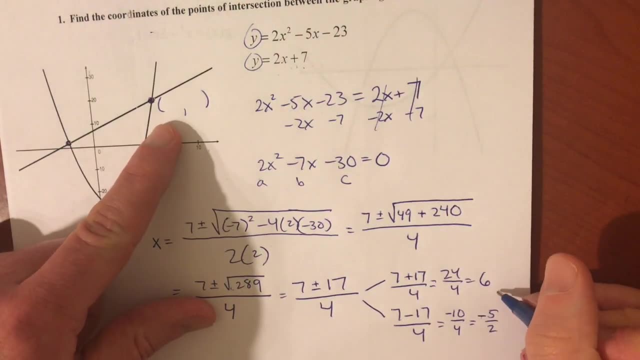 you got to find the x coordinates and the y coordinates. Well, there are two points and I just found the x coordinates for the two points. One of the solutions I got was x equals 6, and that is this one right here, as you can. 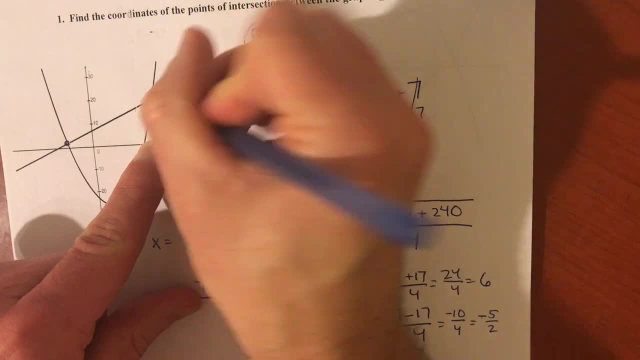 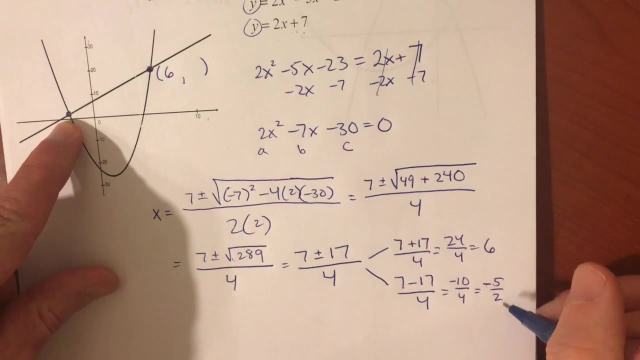 see 0 to 10, and it curves right about there. We didn't know it was going to happen perfectly at 6,, but that seems to make sense. And this one here is going to be negative 6.. Something or other, and that would be negative 2.5, or negative 5, halves comma, something. 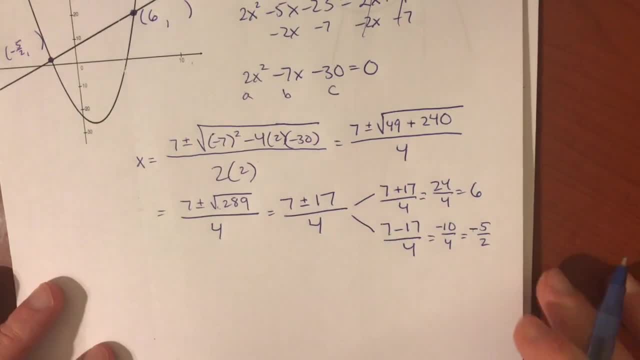 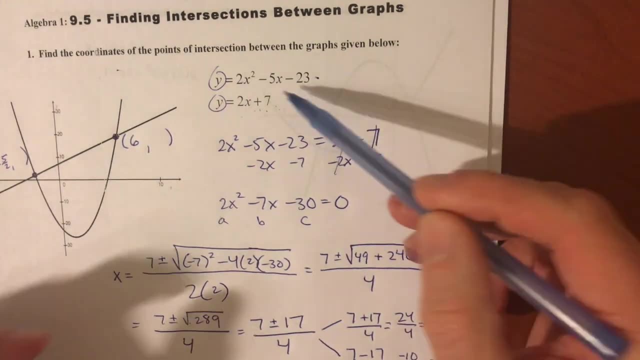 But you got to get the y coordinates. So how do I get the y coordinates? That's easy. Now that you know x, you plug it in. Into which equation? It doesn't matter, because they'll both give you the same values at that point, or they? 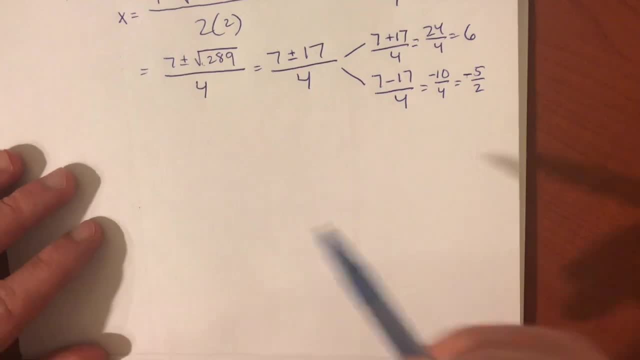 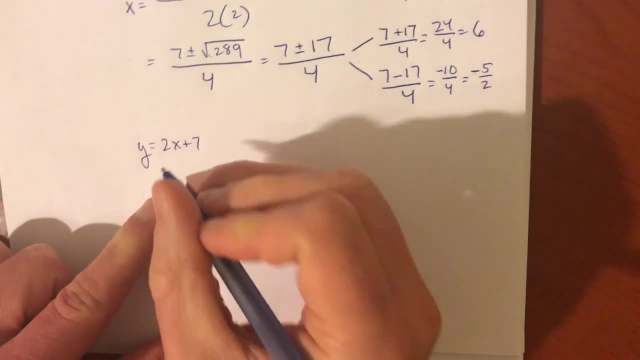 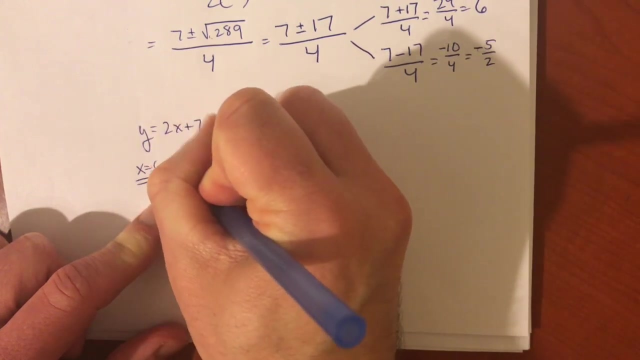 should, if you've done it right. So you can plug into either equation, but I would work with the second one. that's easier to plug, But feel free to do the other. So when x is 6, just be careful. you've got to find the coordinate that goes with that. 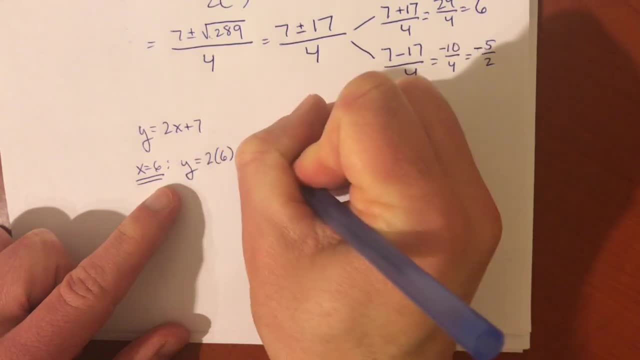 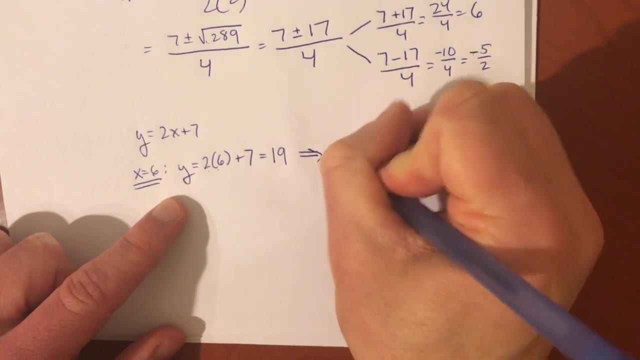 So I'm going to plug 6 in for x and simplify that 2 times 6 is 12, 12 plus 7 is 19.. So one of our points is 6 comma 19,. and that seems to make sense here. 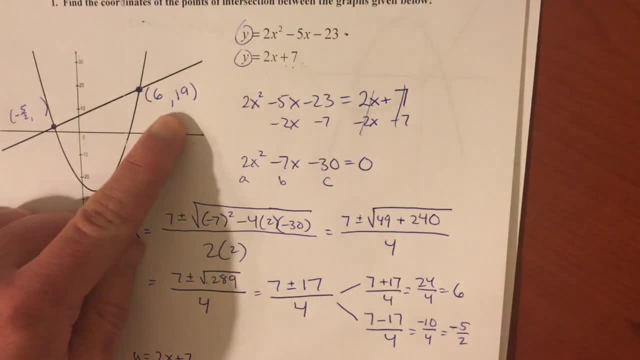 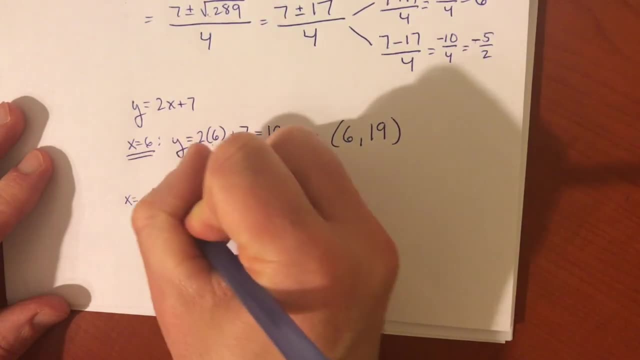 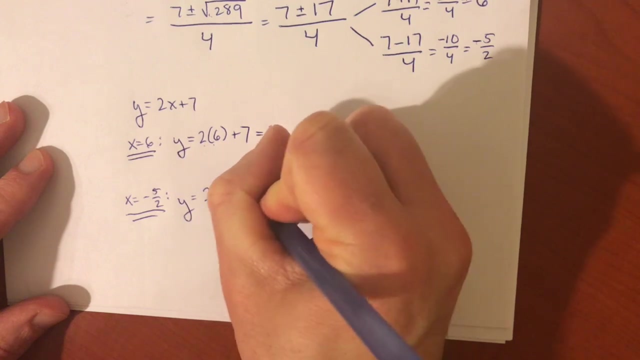 It looks like it's a little bit less than 20, or right around 20.. So it seems good. The other is when x is negative 5 halves or negative 2.5, if you want to use a calculator, I'm going to do this, no calculator. 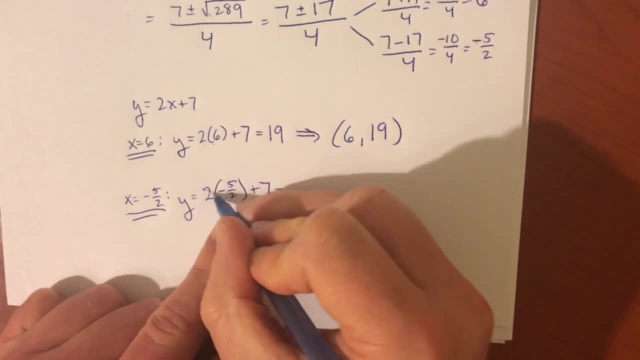 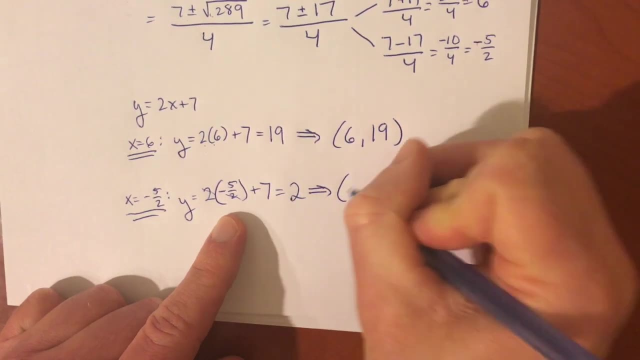 And when you plug that in negative 5 halves times 2, 2's cancel, leaving you with negative 5.. Negative 5 plus 7 is positive 2.. So our other ordered pair is 19.. So that's good. 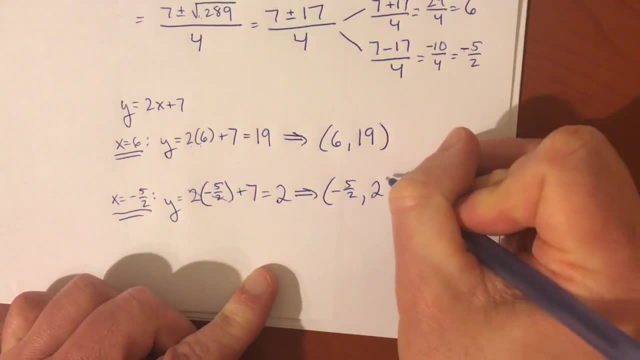 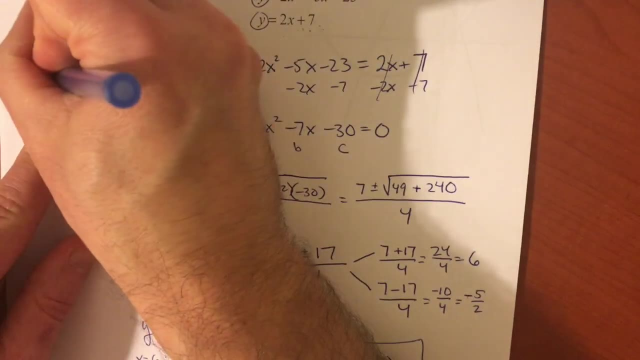 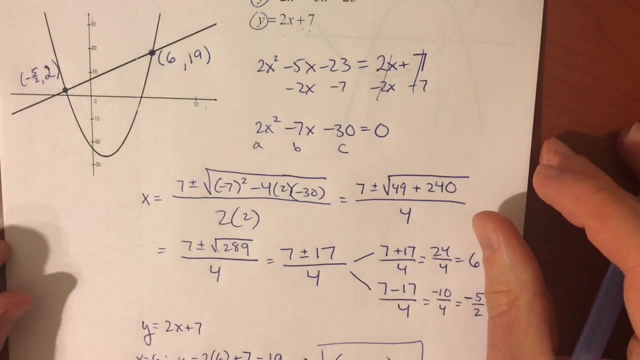 Thank you. Negative 5 halves comma 2.. And those are our two coordinates here and you can also look here. That seems about right that the y coordinate would be positive 2, if that's the scale there. Of course you could check these very easily by just going to Desmos and graphing these. 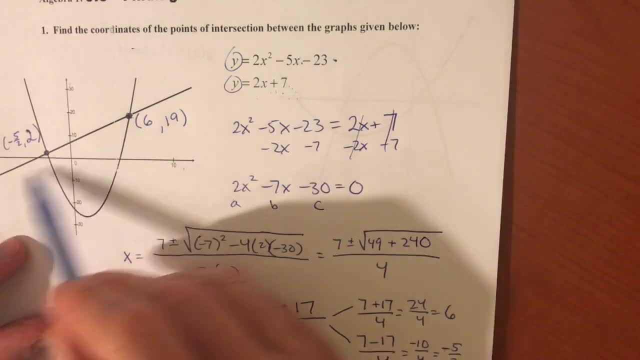 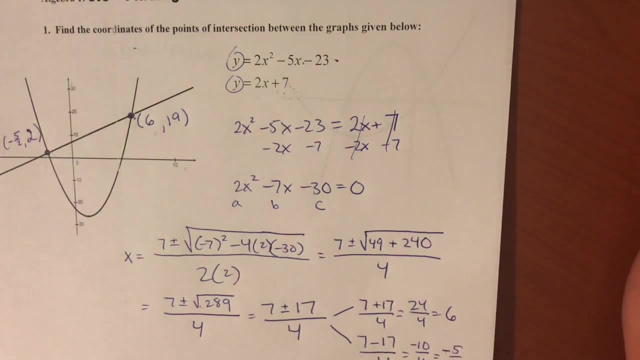 two or any kind of graphing calculator- but Desmos is great at this- Graph these two and then, if you click on them, they're going to highlight those two points And you'll see it's these coordinates exactly. So great way to check yourself. 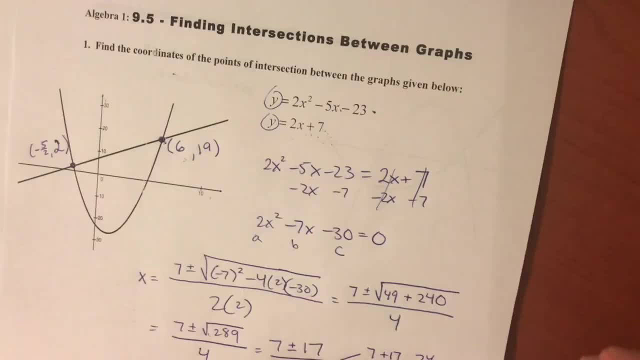 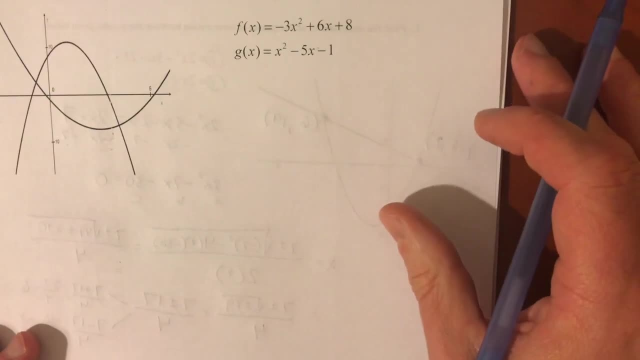 Just don't do the problem with that. You've got to show me the work. And lastly, how about that was the intersection of a line and a parabola? What about the intersection of two different parabolas? It's no big deal. 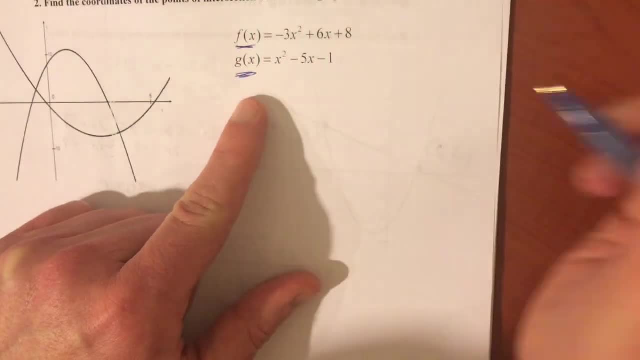 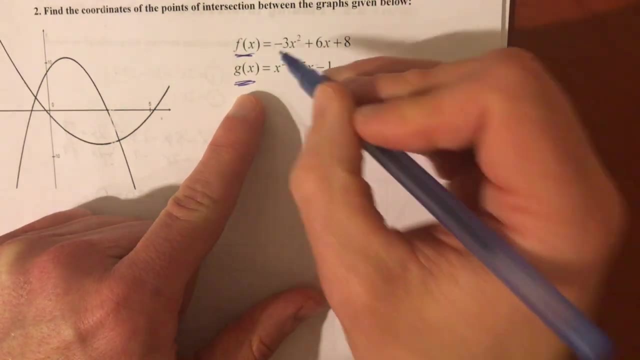 Same exact idea. Instead of y equals, they've used the function notation f of x and g of x. remember, these mean the same thing as y equals, y equals and y equals. So again, I'm really just going to say: if I want to know, when does this graph equal? 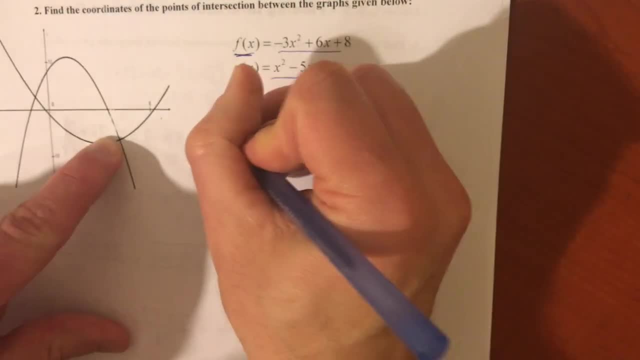 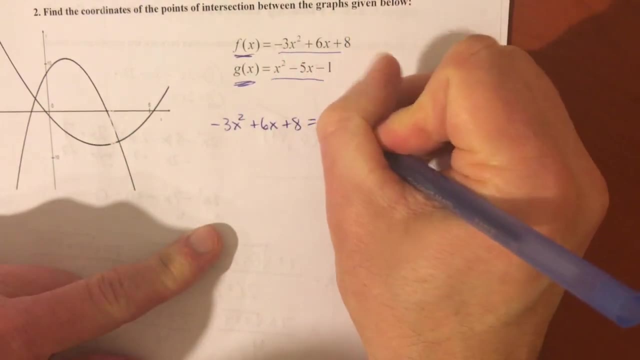 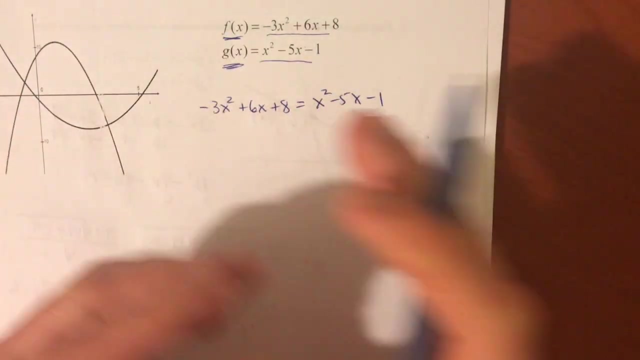 that graph. I'm going to set them equal to each other. So when does negative 3x squared plus 6x plus 8 equal? this other equation of x squared minus 5x minus 1?? Get all of your stuff on one side. make it equal to 0.. 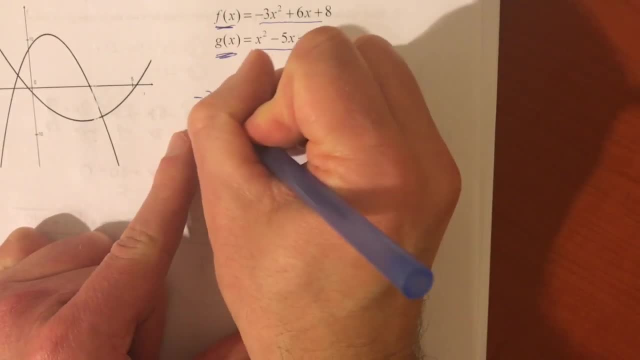 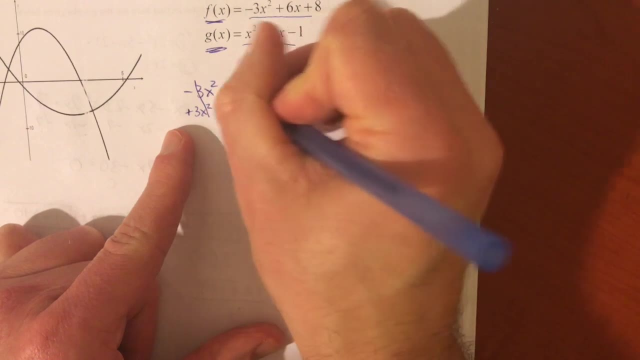 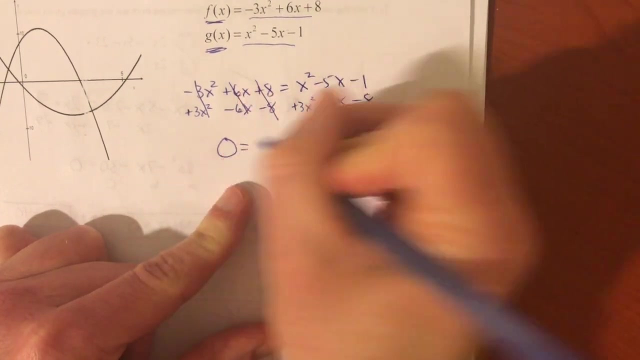 Doesn't matter which side you like to bring it to. I'm going to do that. I'm going to do that. I'm going to bring everything to the right side here. It does not matter. I'm going to add 3x squared. I'm going to subtract 6x, I'm going to subtract 8, and. 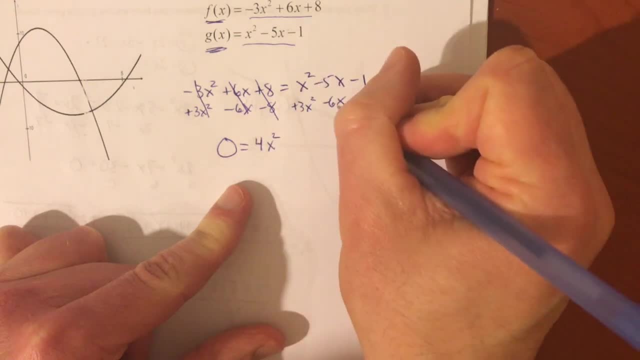 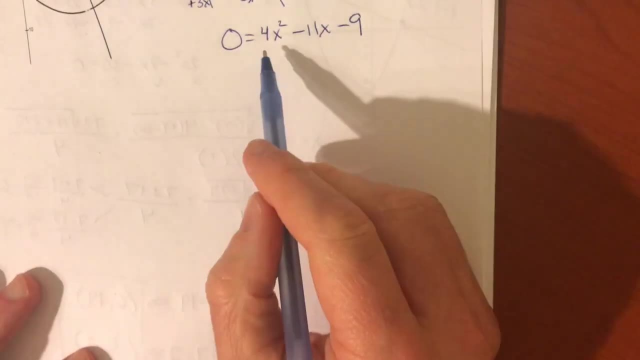 collect all those like terms on this side, That will be 4x squared minus 11x minus 9.. And you could try to factor that if you like, but you probably won't be able to do it at this point because it's only it's got 4 in front of that x squared. 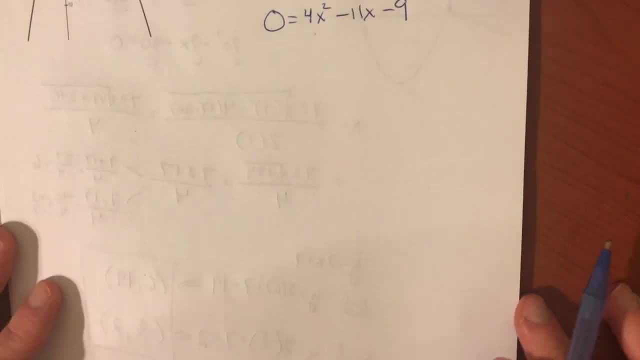 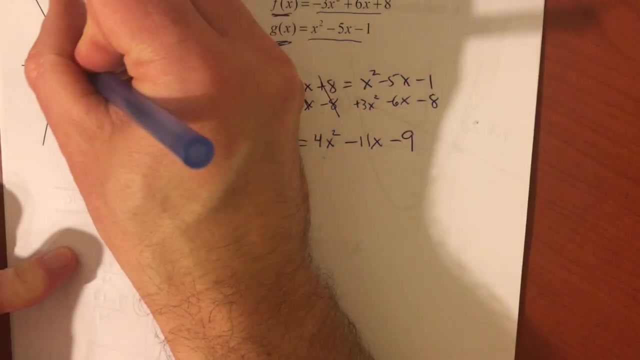 There's no GCF, So let's just use the quadratic formula. That's what it's. that's what's great about it. It works for any quadratic, And I know there have to be two solutions, because I can see there's two intersections. 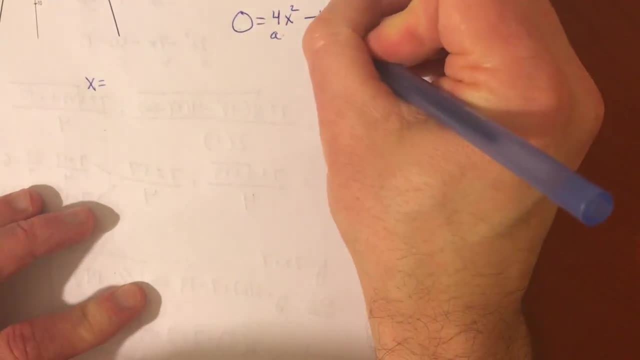 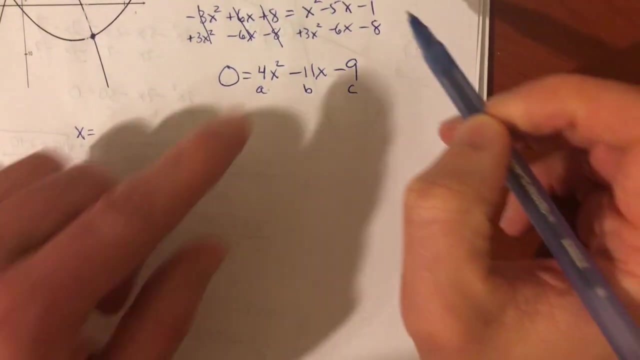 here. So remember, you can't do the quadratic formula until you make it equal to 0, because that's what dictates your a, b and c. And just in case any of you are thinking, well, I was going to bring everything to the 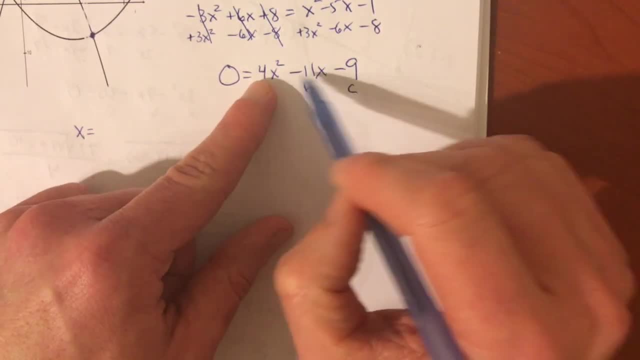 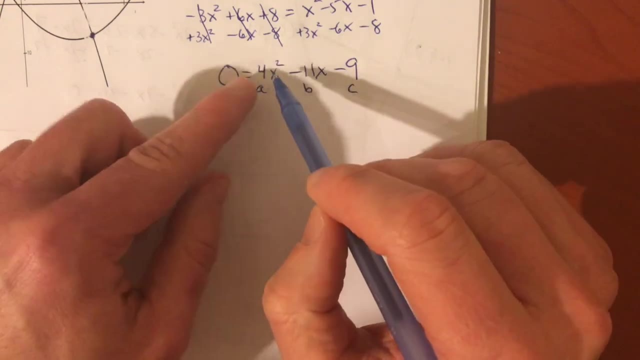 left side of the equation. You would have had the almost identical equations available. You would have had the almost identical equations available. You would have had this: you would have had negative 4x squared plus 11x plus 9.. You would have had. just all the signs were opposite. 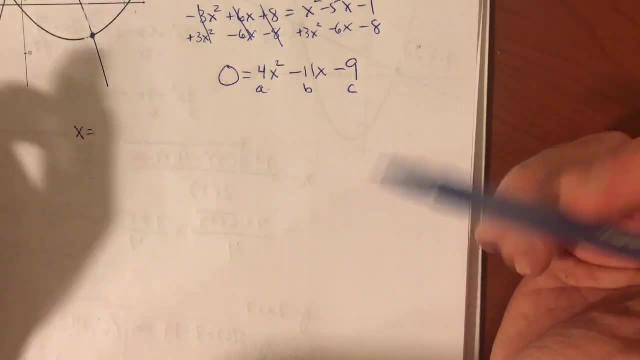 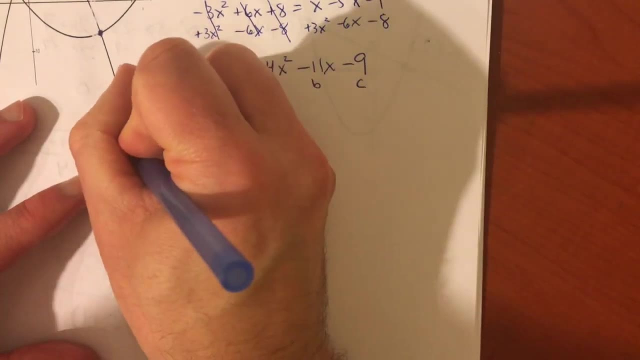 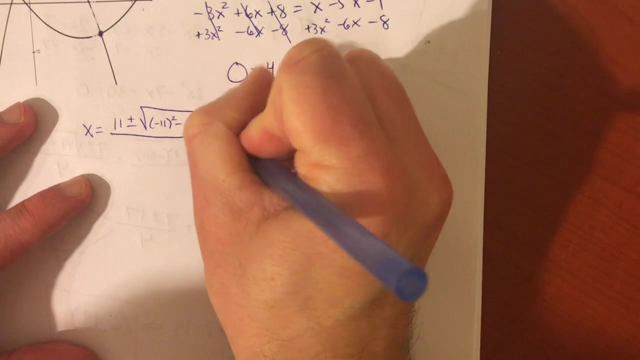 And when you do the quadratic formula, everything will work out the same in the end. So it does not matter as long as one side is 0.. So here we go. X is equal to negative b plus or minus the square root of b squared minus 4ac all over. 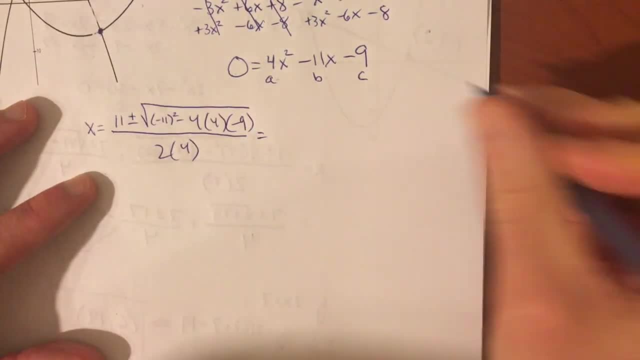 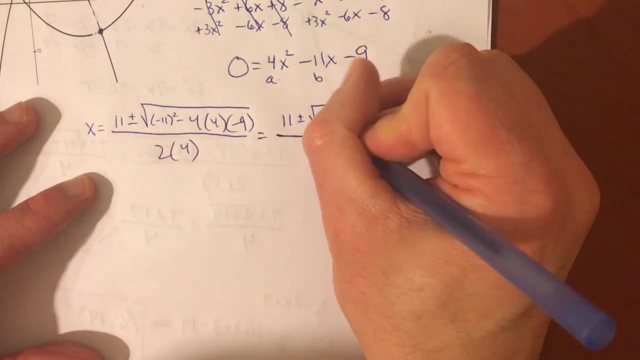 2a, And here we go. Thank you, Mrs Hammond. Let's just simplify here: 11 plus or minus the square root of 11, negative, 11 squared positive: 121, negative times. positive times negative. That's a positive. 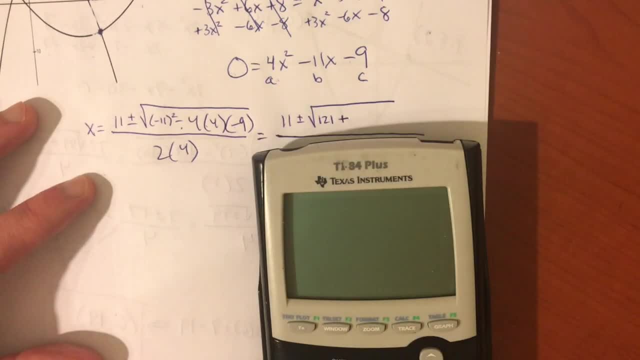 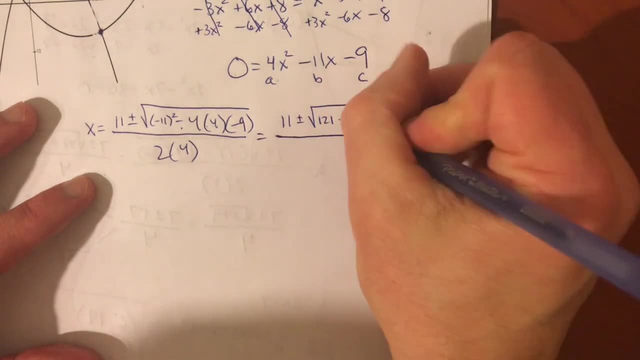 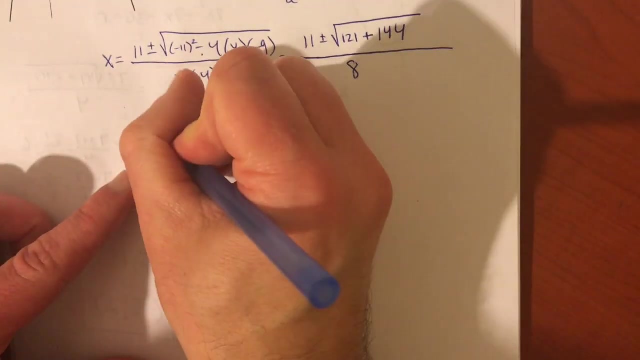 And 4 times 4 times 9,- eh, I'm going to cheat a little bit, feeling lazy today. That's 16 times 9.. That's 144.. I could have done that, but I'm getting old And simplify this. on the inside, 121 plus 144. 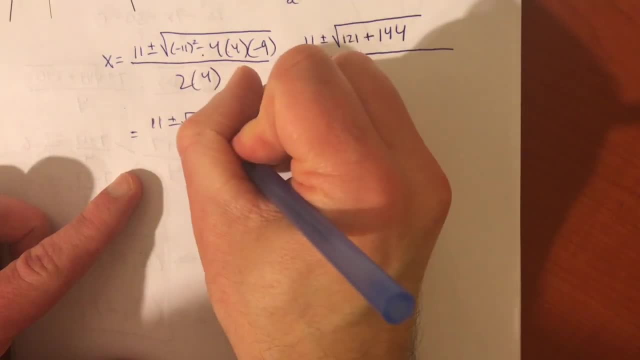 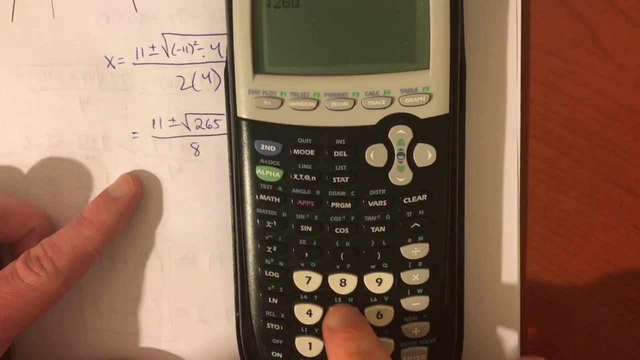 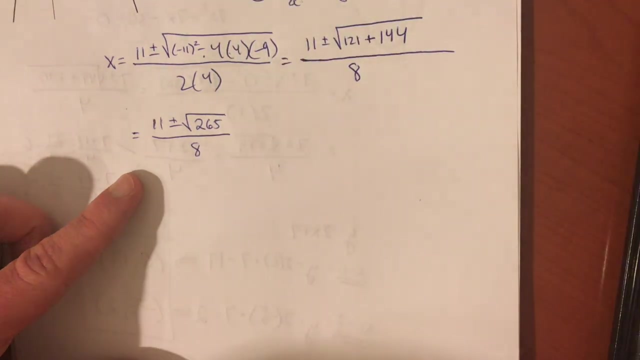 That is going to be 265.. And 265 is not a perfect square, I can tell you, but don't believe me. Here we go, We get about 16.28.. That's where we've been rounding it to the nearest hundredth. 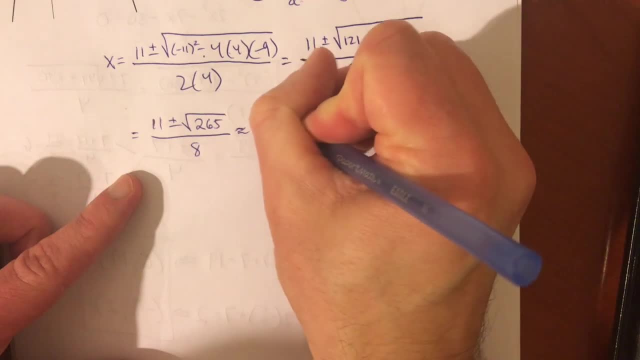 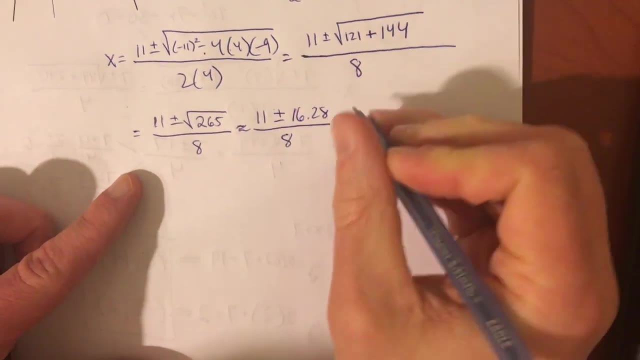 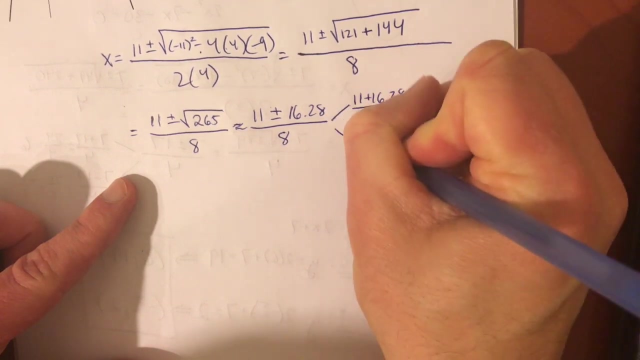 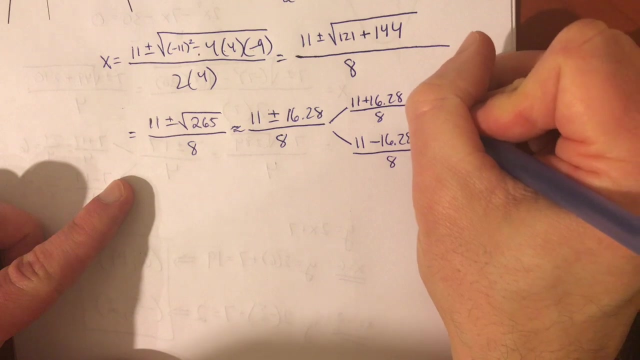 There we go. That's a perfect square. So that's approximately 11 plus or minus 16.28, all divided by 8.. And just be careful handling that plus or minus. It's two separate values: 11 plus 16.28 over 8,, 11 minus 16.28 over 8.. 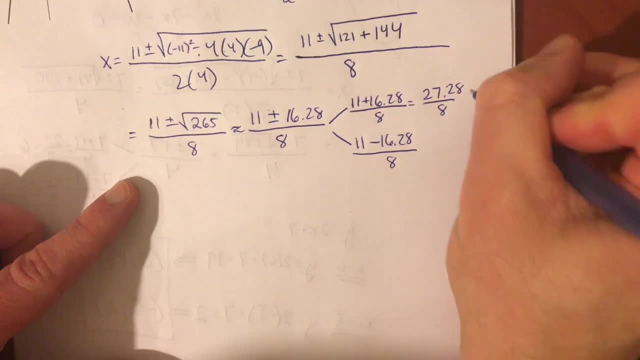 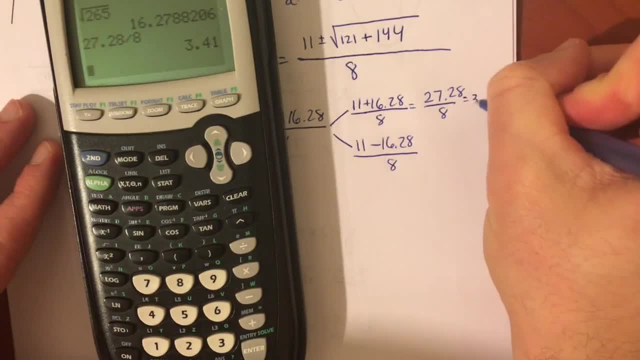 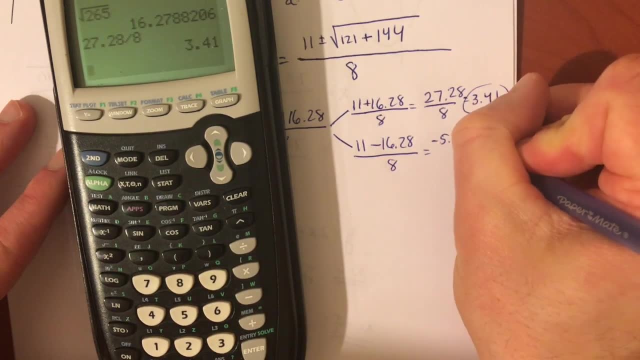 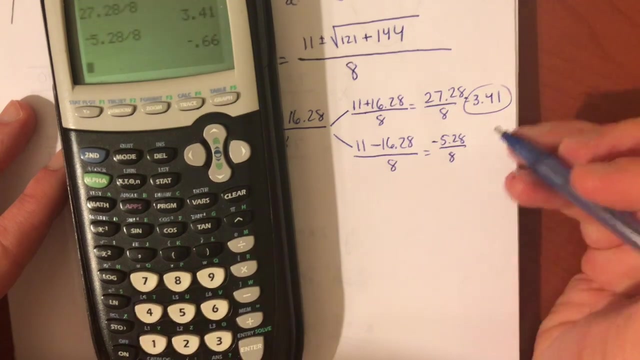 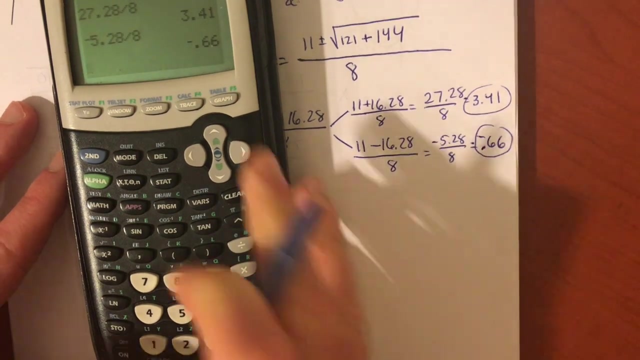 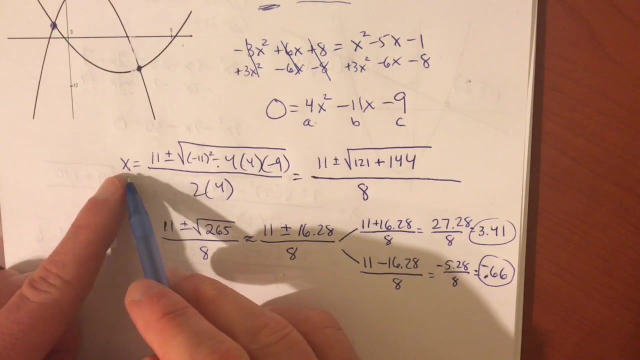 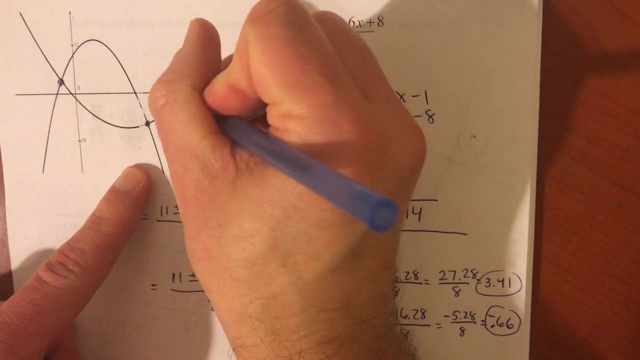 That divided by 8. It will give you about 47. 67.28. x values for the points of intersection. that's what you're solving for when you do the quadratic formula, the x values, and this one is at 3.41, and that seems about right because look at this x scale. 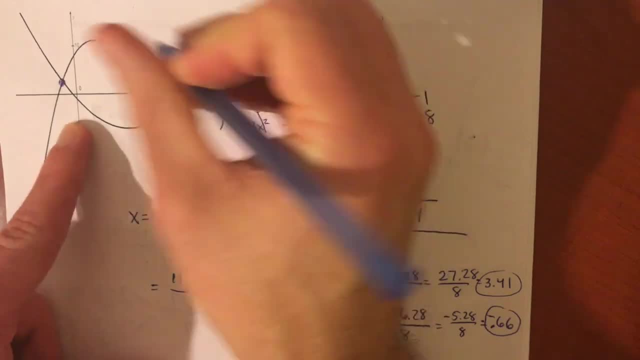 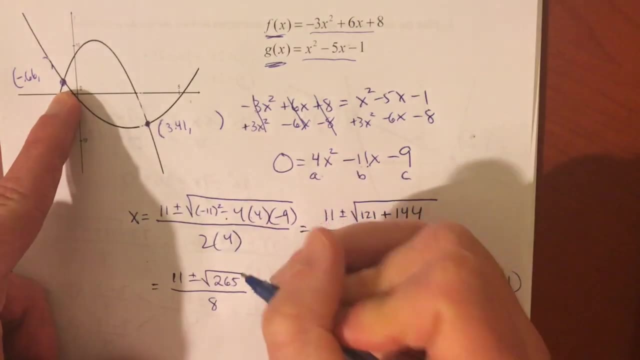 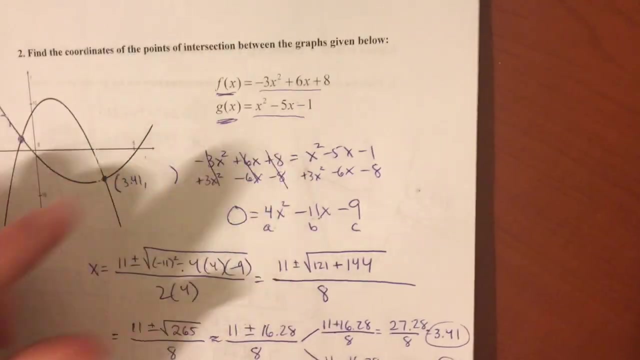 that's five, so 3.41 seems about right and that means this is a really small value and that's negative 0.66. it's got a positive y value and this one's got a negative y value. now to plug those in which equation? yeah, it's about a toss-up, i'll go into g. 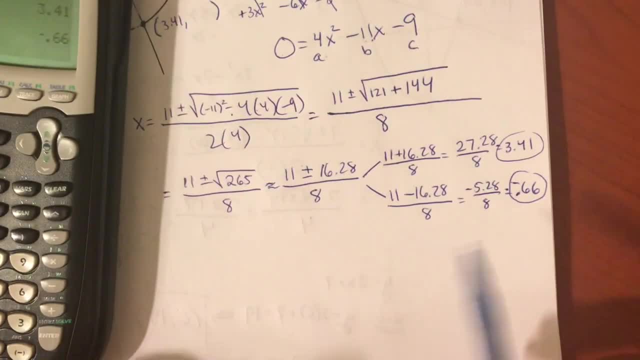 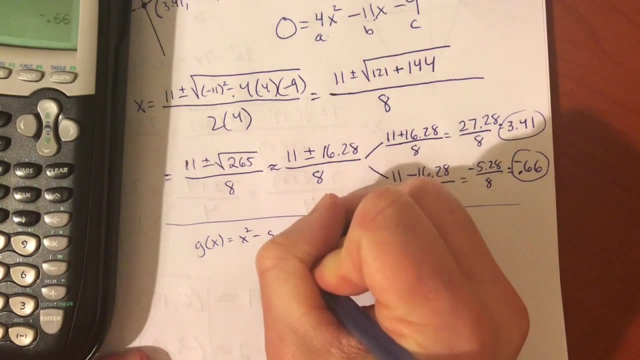 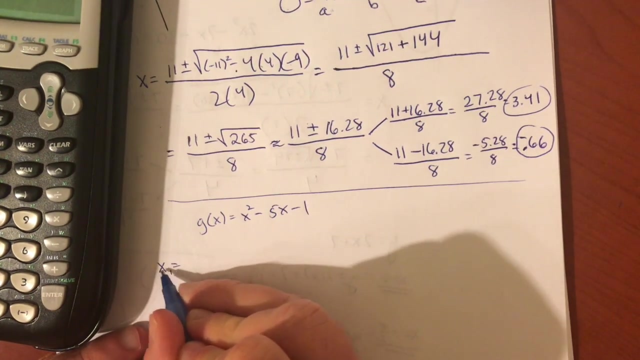 seems like it's slightly easier, but it's about the same amount of work. so g of x is x squared minus 5, x minus 1 and our first x value. sometimes people write this to distinguish. they write: x sub 1 is 3.41. 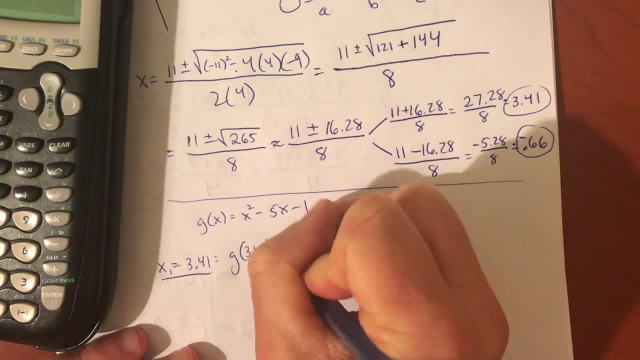 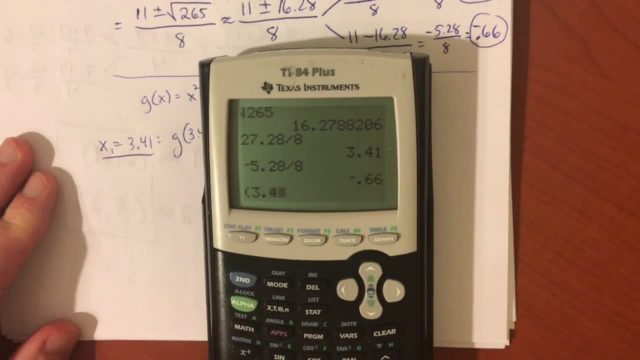 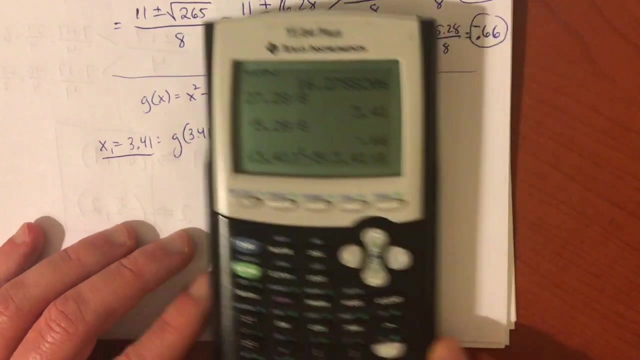 and when i plug that into g, g of 3.41 is definitely going to be careful and use my calculator here with these parentheses: 3.41 squared minus 5 times 3.41 minus 1, you get about negative 6.42. 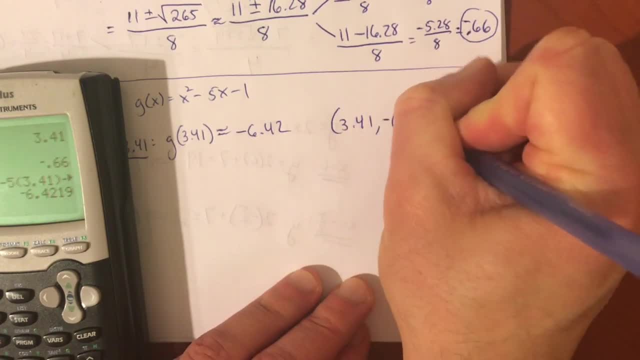 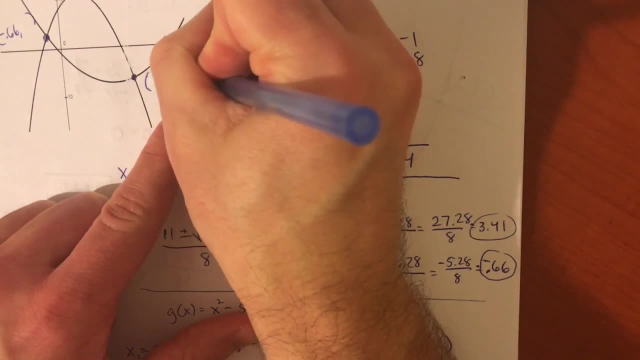 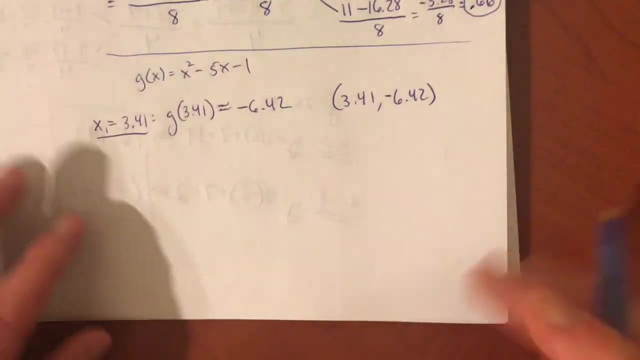 and so that is one of the points. 3.41, negative 6.42. we said that seems like it should have a negative y value and we can check that y scale. that seems about right. if that's negative, 10, that seems about negative. 6.42, the other x value, or x sub 2 if you want the second. 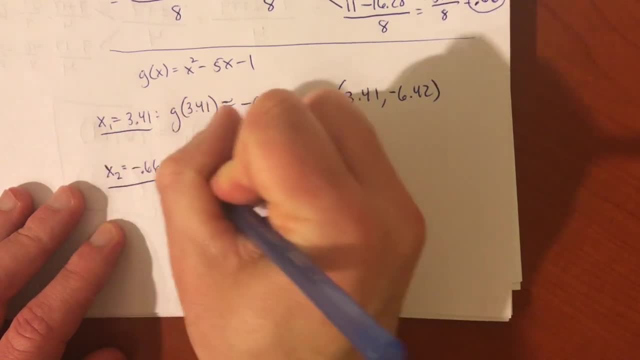 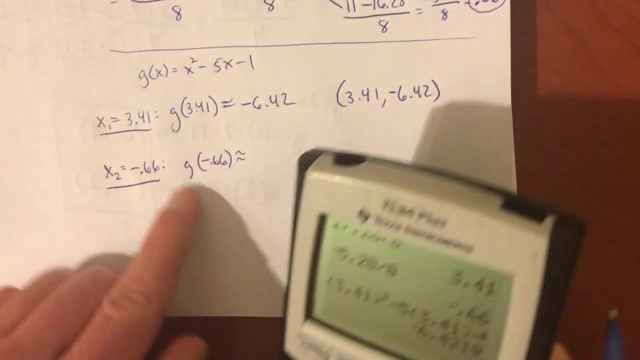 x value was negative, 0.66. i'm going to plug that into g or f again, it shouldn't matter. or if you want to plug it into f and make sure you get the same value you get from g. that would be one way to check yourself. 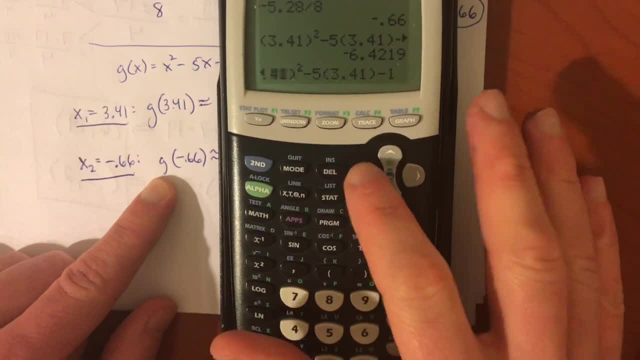 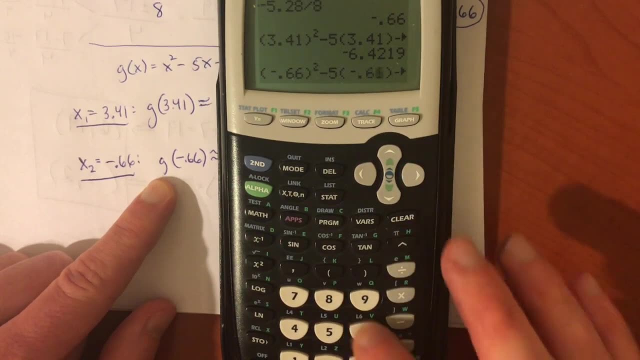 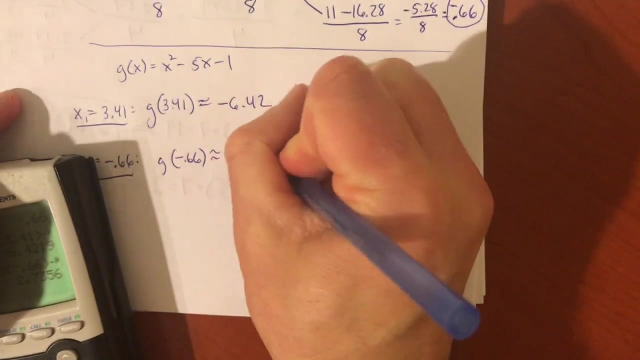 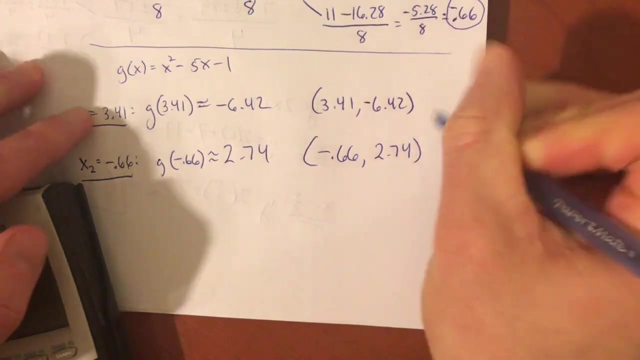 i'll just bring back the last equation and plug in negative 0.66, change that to and you get about 2.74. so the other point of intersection is about negative 0.66, 2.7, 4.34. And there you go, kids, Check out that graph. Go check it on Desmos if you like. 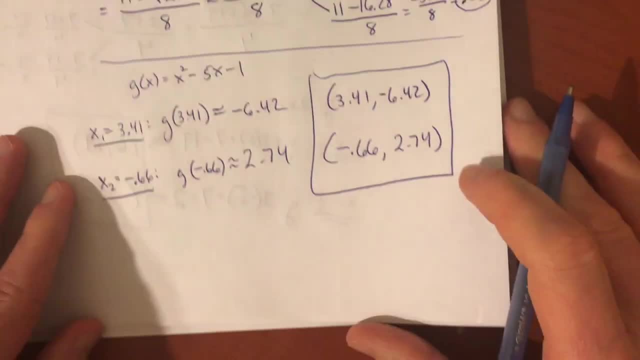 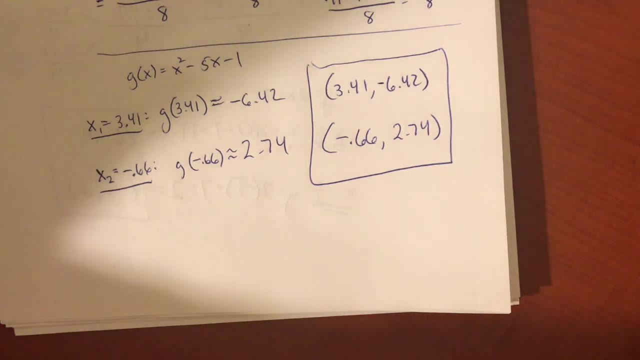 And you're good to go there. That seems about right And there's your solution. You got any trouble? email me, check Desmos, but do the work yourselves. 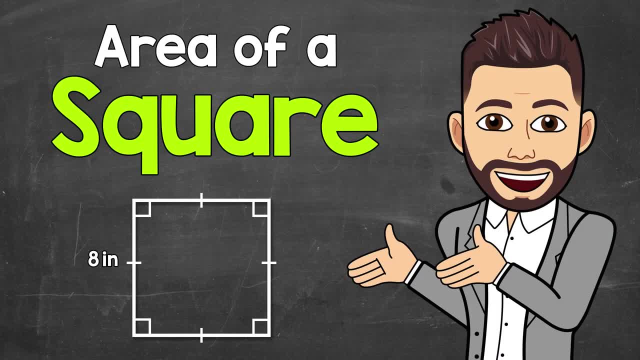 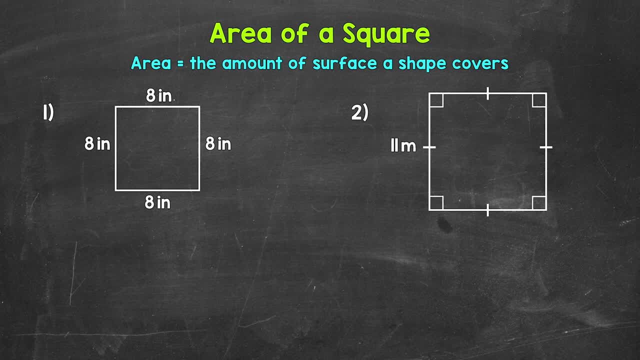 Welcome to Math with Mr J. In this video I'm going to cover how to find the area of a square. Now remember, area is the amount of surface a shape covers. Let's jump into our examples, starting with number one, where we need to find the area of that square.